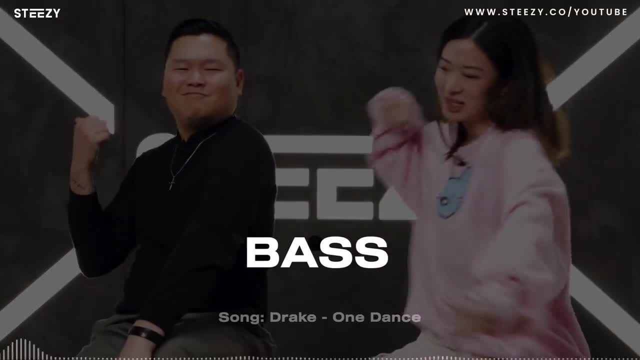 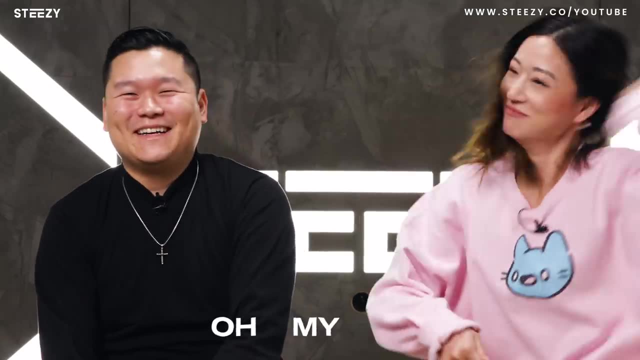 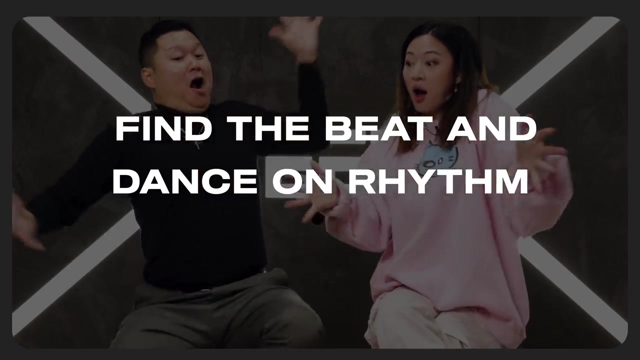 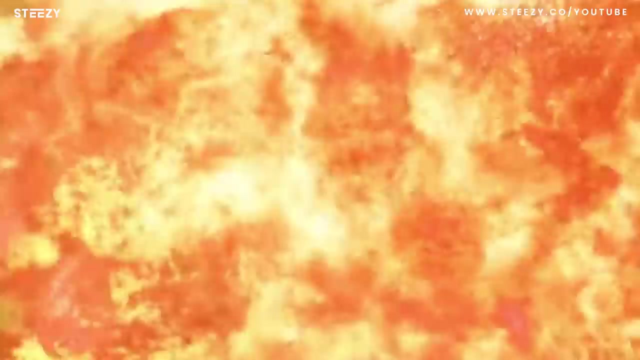 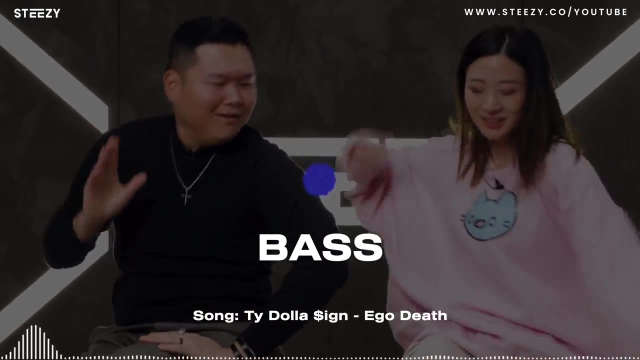 Let's find the beat of this song. Many hours later, I think we found it. You hear that The, what, The, The, what, The. Now let's listen to the same in a different song. You hear that Nice, Last one. 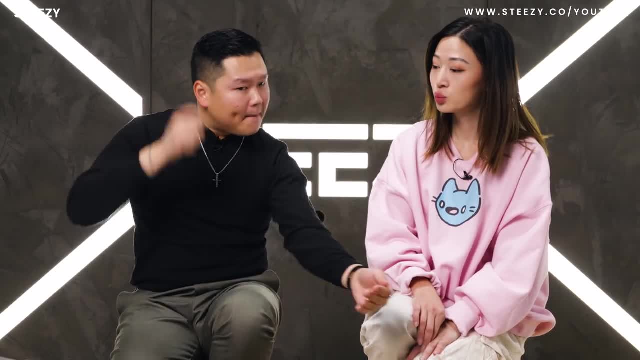 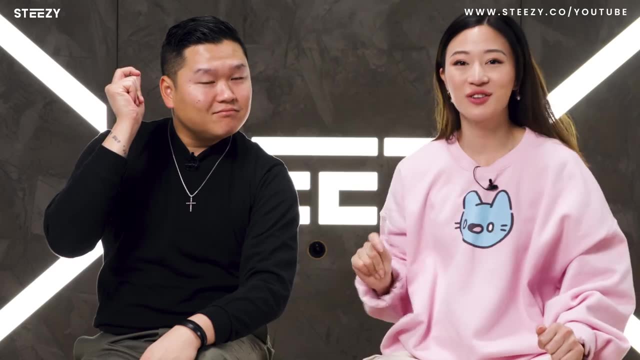 Okay, now we're going to look for the snare sound. It can also sound like or like It's kind of a sharp or staccato sound. Now I want you to either clap or snap when you hear the sound. Let's try this on every even number. 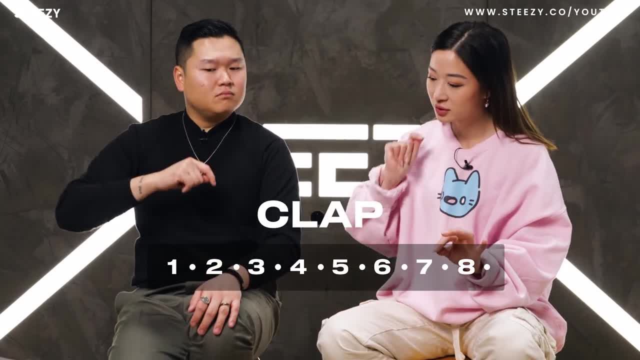 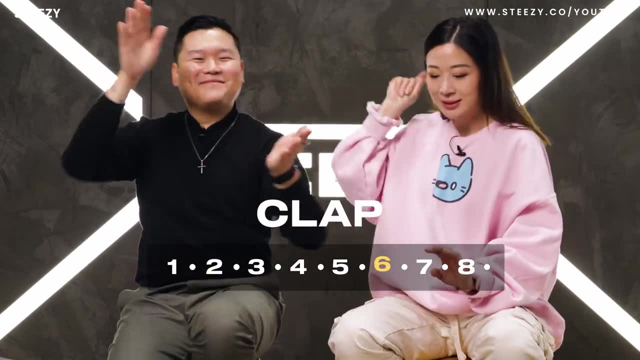 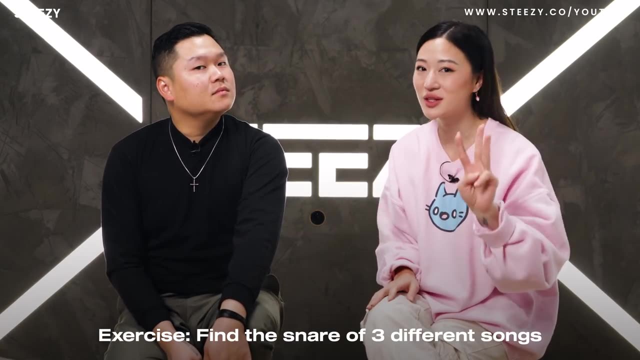 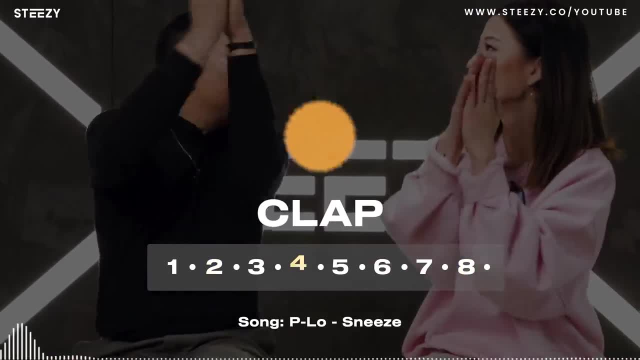 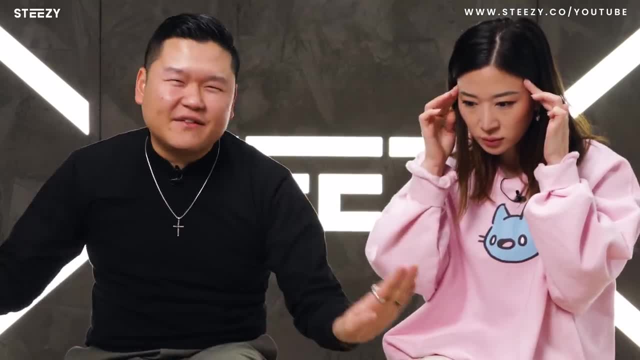 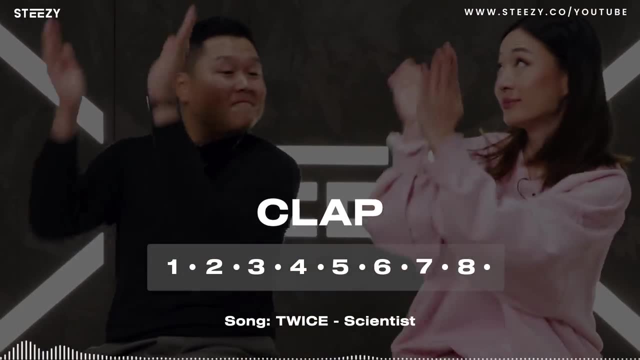 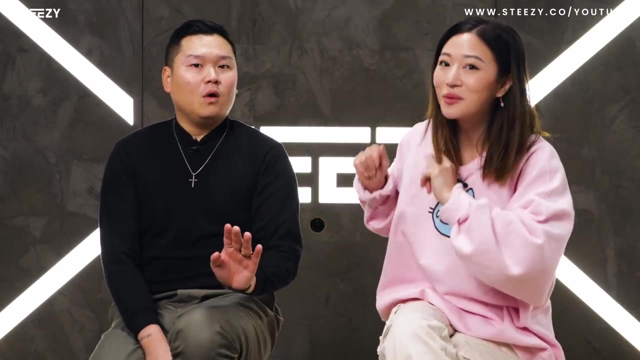 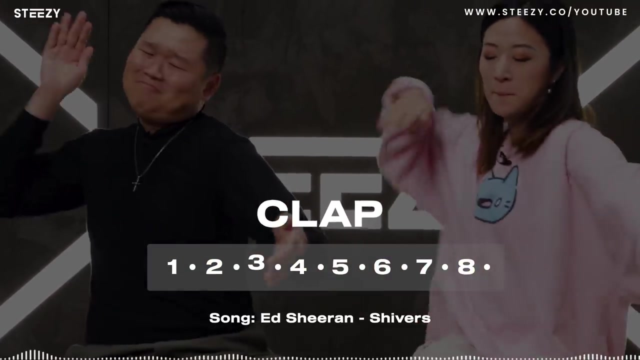 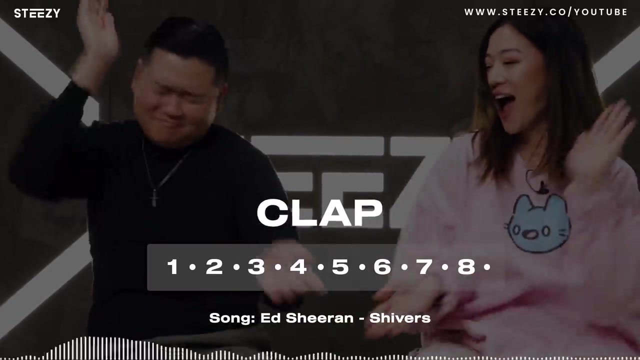 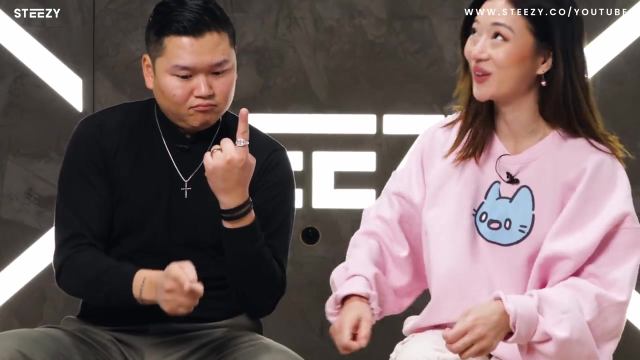 1, 2,, 3, 4. 1,, 2,, 3, 4. Focus on that sharp sound and forget everything else. Last one: This one is gonna have a little spice, so watch out. We just used two different elements of music, either the bass or the snare, to mark the rhythm. 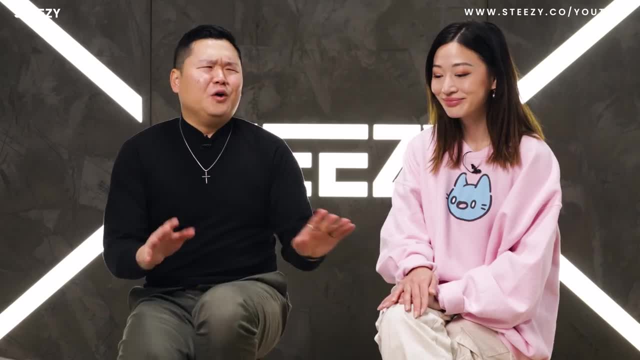 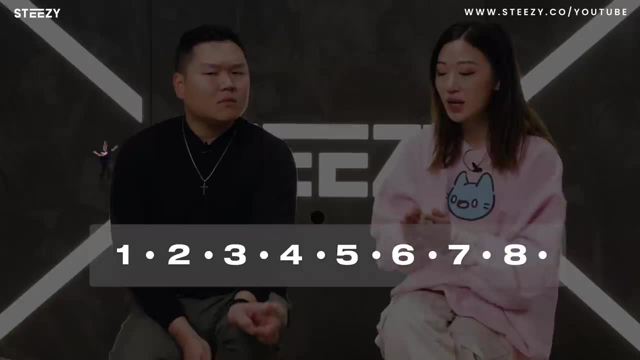 You can use these two sounds to find the beat for a lot of different kinds of music. So we were just clapping. That's the easy part. The hard part is actually dancing on beat. One of the reasons this is difficult is because the time in between the music markers doesn't change. 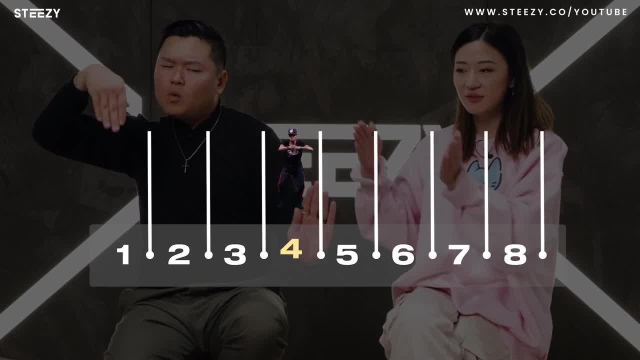 But when you're dancing, you're doing different types of motions that all have to fit in the same amount of time, Meaning you have to use different amounts of time. Meaning you have to use different amounts of time. You have to use different amounts of energy in order to stay on beat. 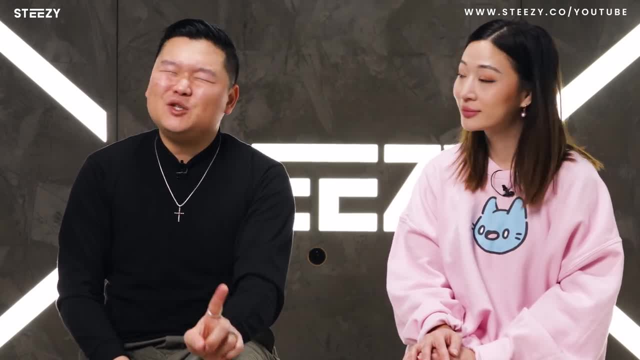 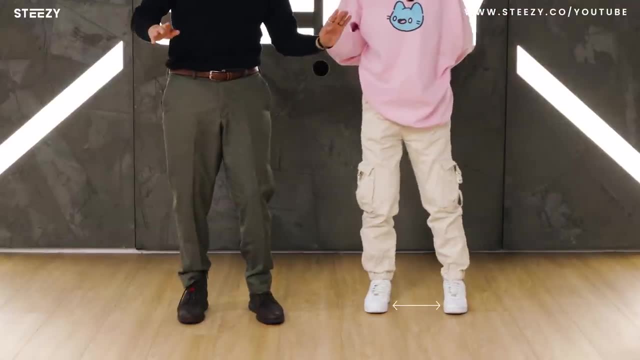 So, to practice staying on rhythm, we're gonna do one last little exercise, but doing a little bit of dancing, Let's go. You're gonna start with any leg, It doesn't matter, We're gonna take a small step out and take a small step together. 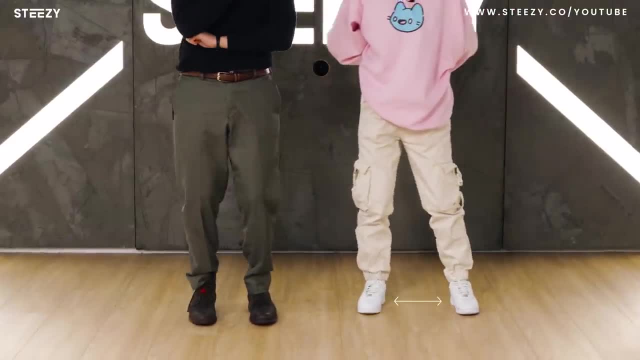 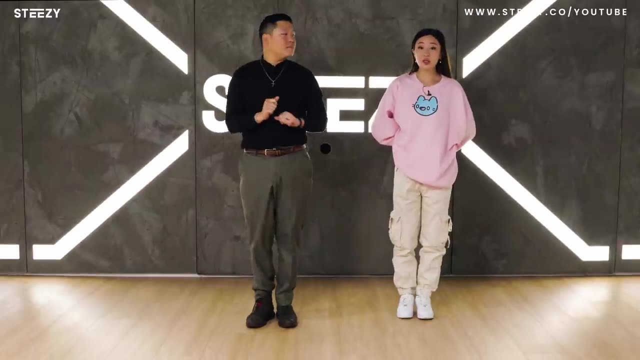 Small step out, small step together. Again, small out together, out together. Last time out together, out together. And then we're gonna do the same thing, but we're gonna do a bigger step. Ready? Five, six, seven. 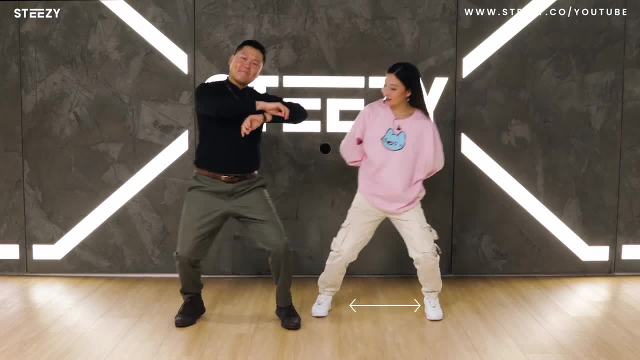 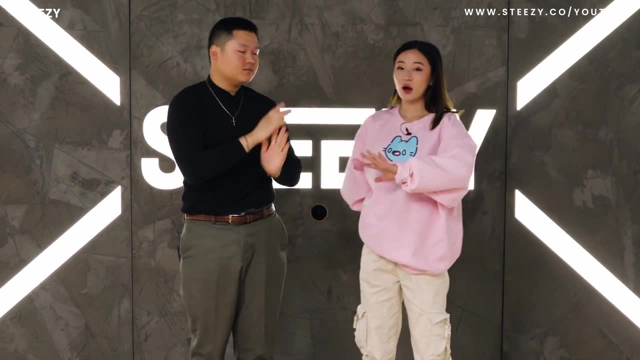 Big step: out together, out together, Again. out together, out together. One more time Out together and good. So in order to practice staying on rhythm while we're doing different sizes of movement, we're gonna do an eight count. 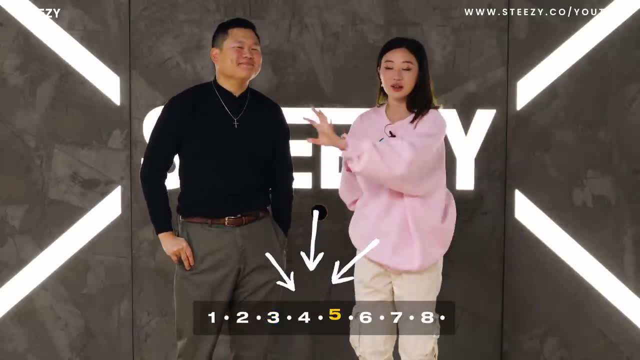 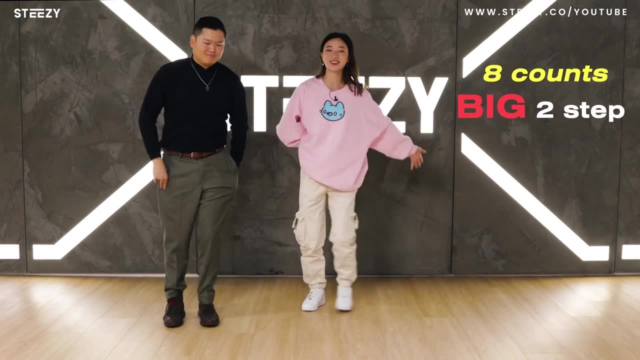 So don't worry about counting, We'll count for you and you'll see it on the screen. We're gonna do an eight count of small together out together. small together out together. big together out together. big together out together. 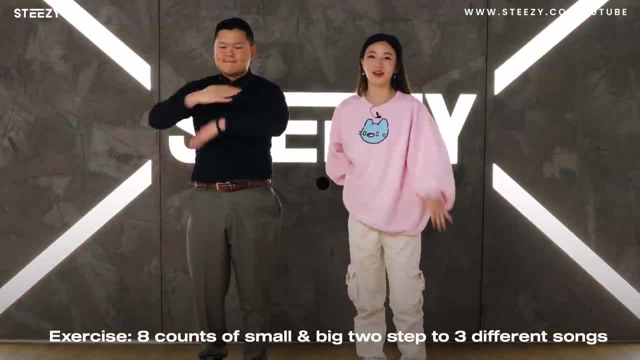 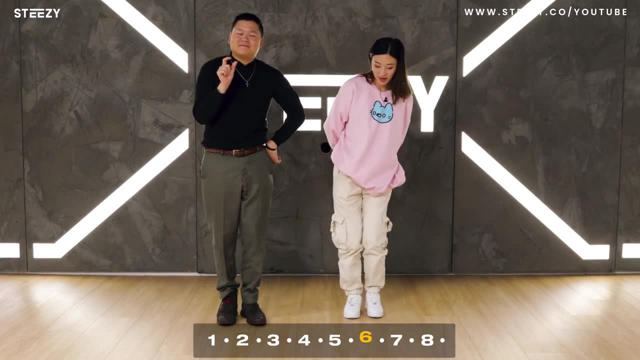 We're gonna try this to the three songs we heard at the beginning of this video. Just follow along, Baby. I like you so Small, small and big. Let's go Grips on your waist front way back way. 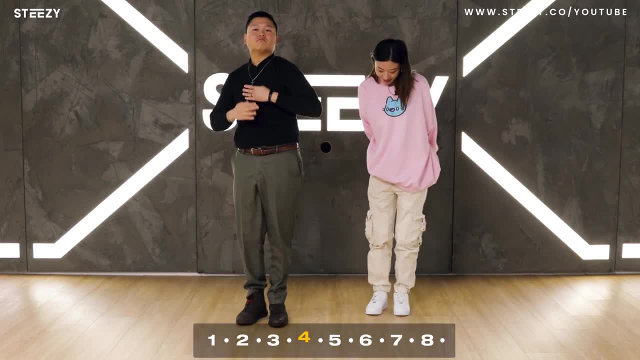 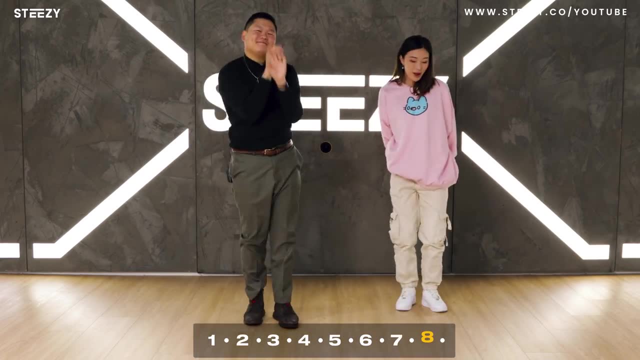 You know that I don't play Streets- not safe. but I never run away, Even when I'm away, OT, OT. there's never much love when we go OT. I pray to make it back in one piece And five, six good. 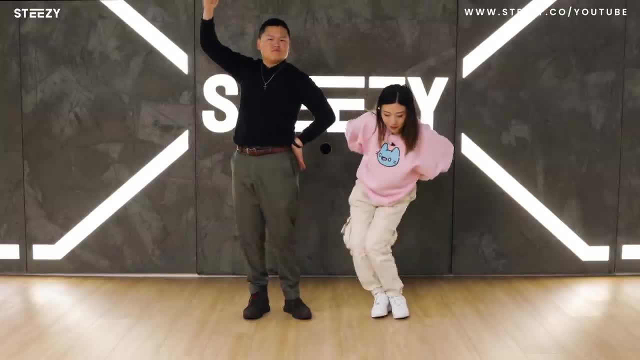 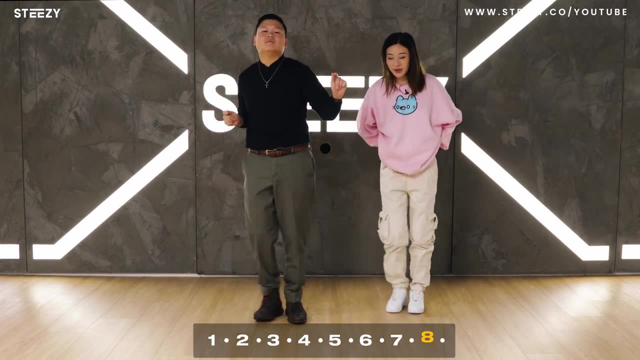 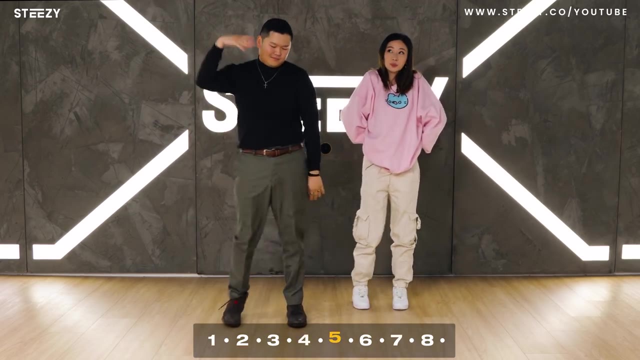 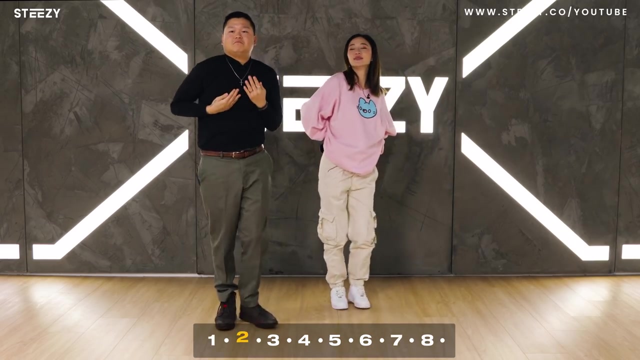 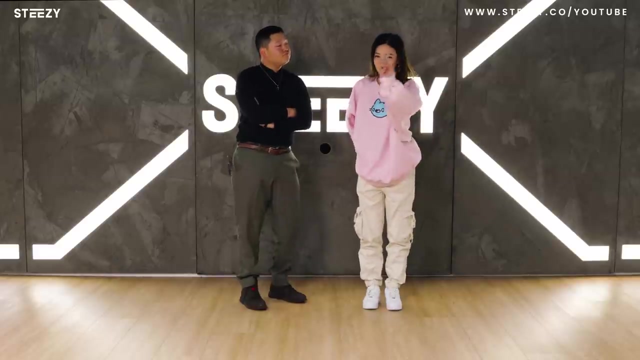 Good job. One, two, three, four and five, six. Start on one: Small in small in small And big And small. Last time, small Good job. Last song. we're gonna start on the one.